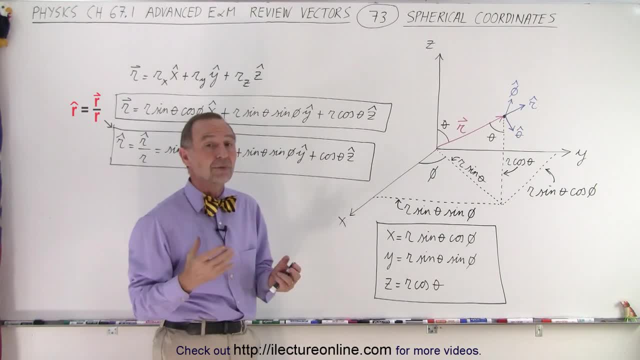 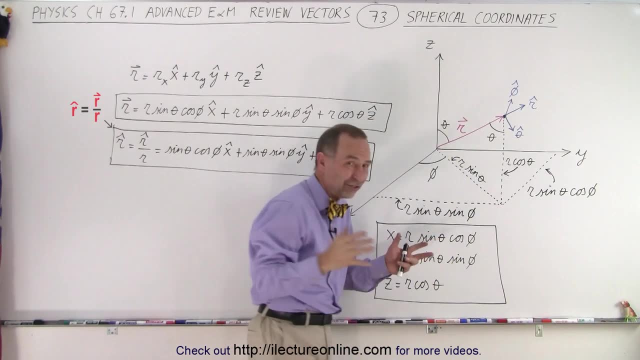 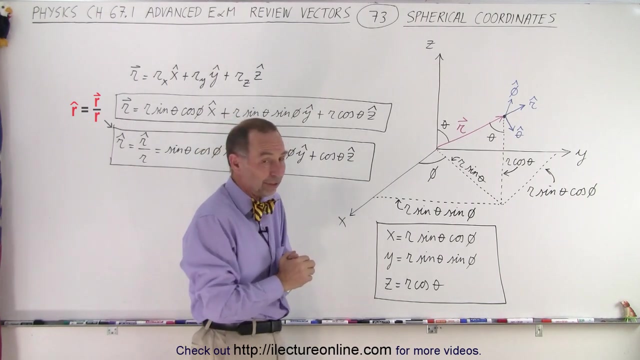 But it does make sense when we start working out problems that by standard notation we simply take the origin of the vector, the position vector r, because essentially r stands for the position vector. Well, we simply start with the tail at the origin. It just makes sense as a reference point. It normally doesn't have to be that way. 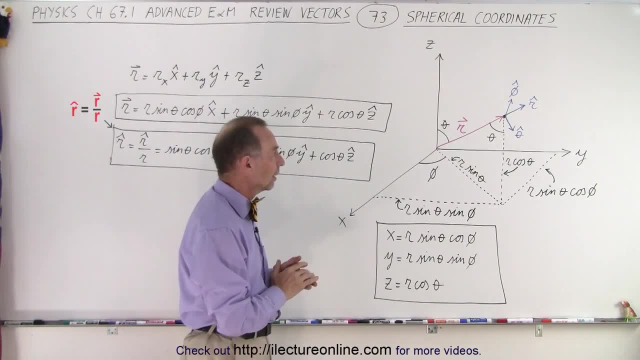 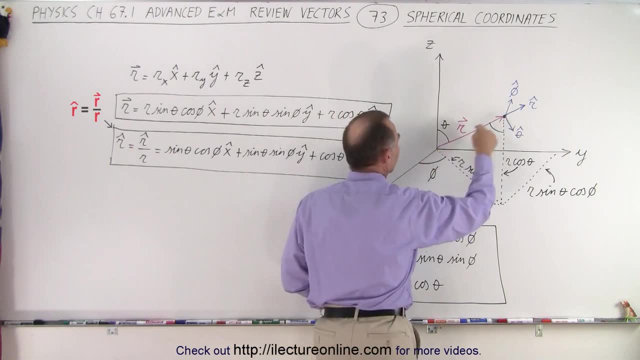 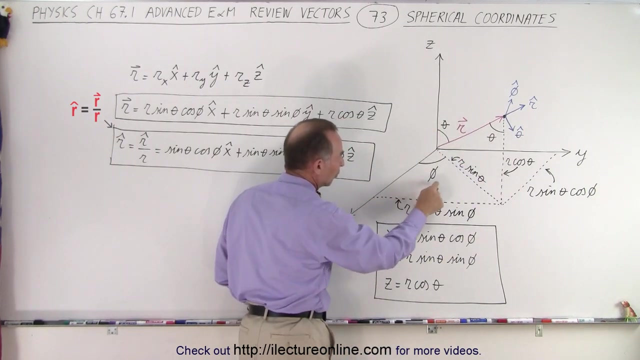 but we simply do that so that things make a little bit more sense. So notice, we have three components. We have the length of the vector r, we have the angle along the xy plane relative to the x-axis- We call that the angle phi- And then we have the angle to the. 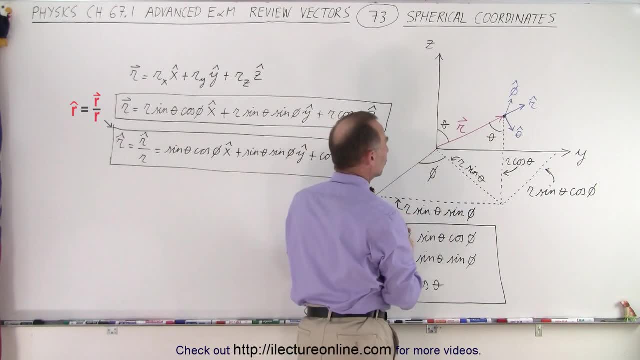 vector r relative to the z-axis. So notice that here we have the vector r. It can be positioned in any direction. It's simply the angle from the z-axis to the vector r. no matter which way vector r is pointed, That angle is called the angle theta. And then, if you see the projection of the, 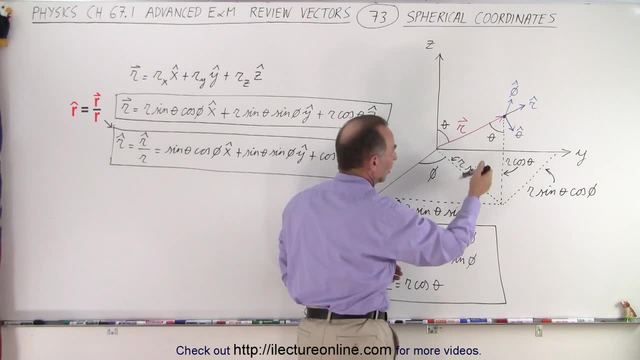 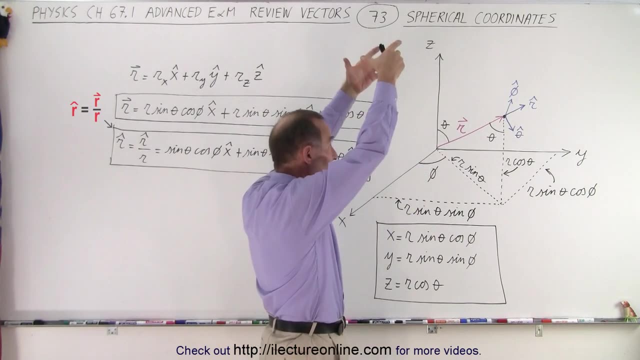 vector r onto the xy plane, which is this dotted line right here. So we essentially, if we have light shining from above, from the z-axis, from a point in the z direction, along the z-axis straight down, then the shadow of the r vector would be this line right. 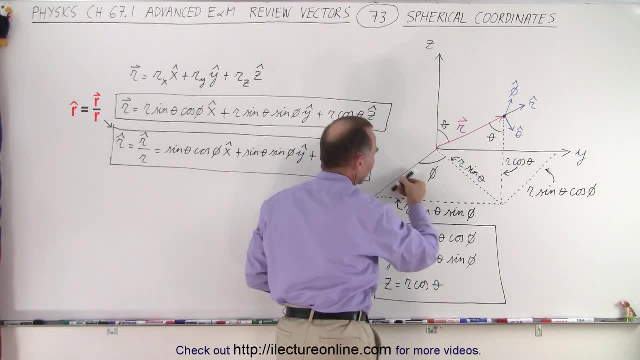 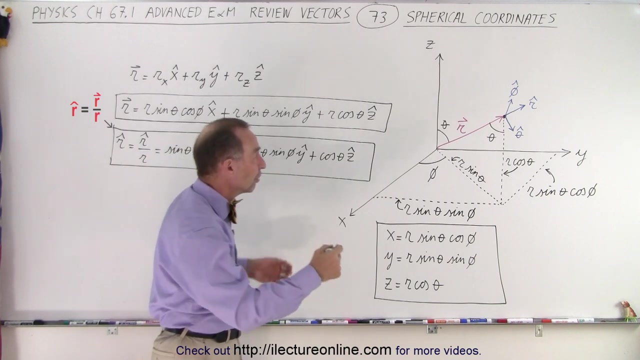 here And you can see that the angle of that line relative, that's the projection of the r vector onto the xy plane, from that line to the x-axis, that angle right here is considered the angle phi. So we tend to represent everything in space in spherical coordinates in terms 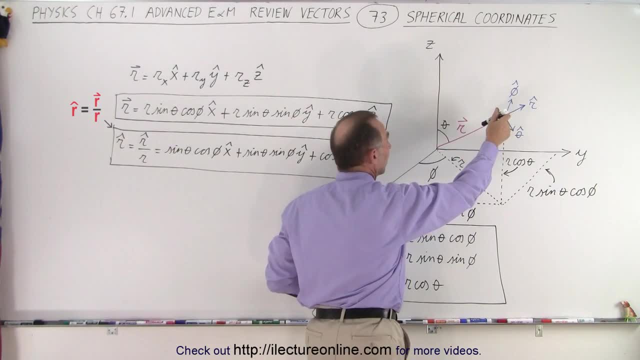 of how far away from the origin. that's the magnitude r. That point, if we draw a vector from the origin to there and that line, the line between the z-axis and that vector r, that angle is theta. And then the projection of r onto the xy plane, the angle between that line. 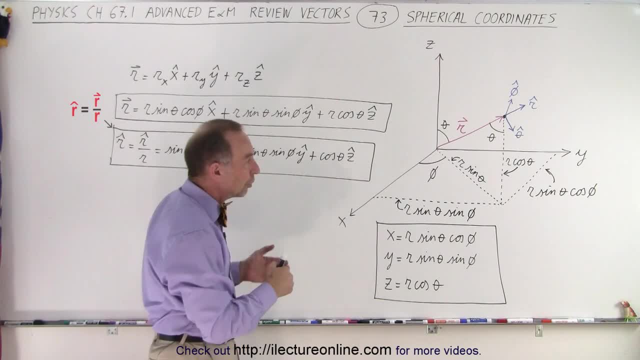 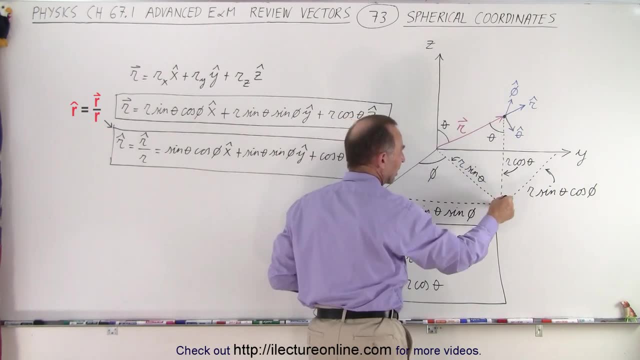 and the x-axis is the angle phi. Now, how do we represent the distances? So notice, if I take this point right here and I project it straight down onto the xy plane, this point right here, there's a certain distance away from that point to the xy plane. that's the z-axis, and so that's. 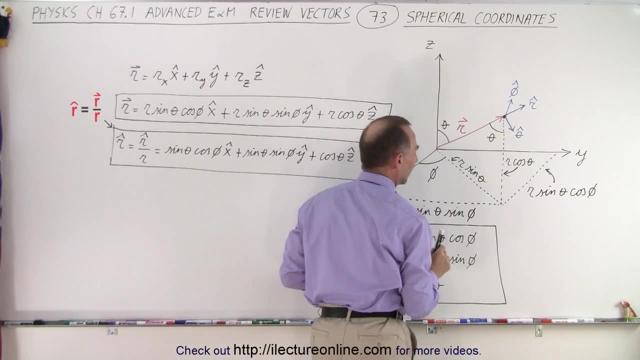 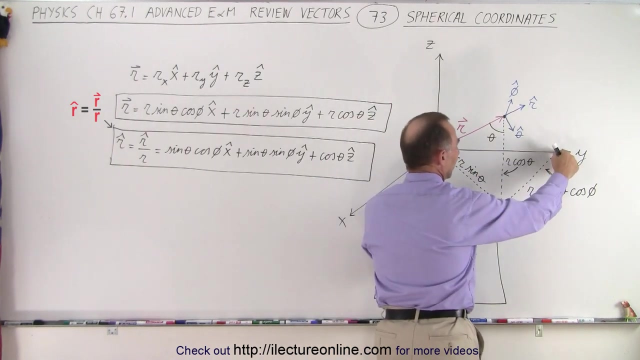 the distance in the z direction from the xy plane to the point. Then we have the distance from that point, a projection straight down to the xy plane, from there to the x-axis and the distance from there to the y-axis. Notice that this represents the y-coordinate of that point. this represents: 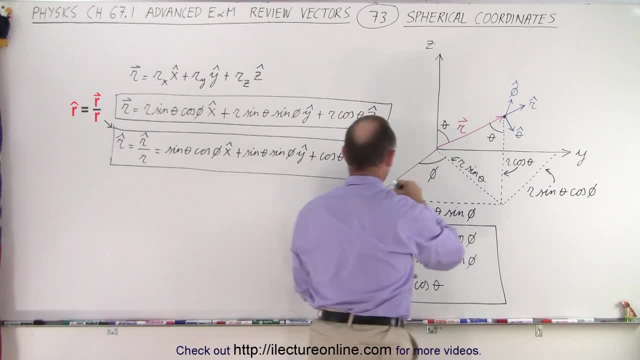 the x-coordinate of that point, the distance from the origin to the point along the x-axis where that point is located, the distance from the origin to the point along the y-axis where that's located. So here we have the y-distance, we have the x-distance. 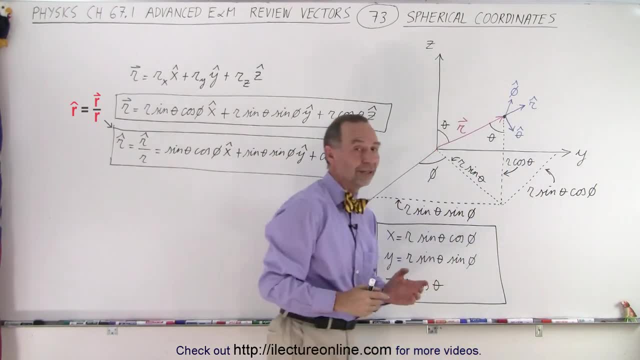 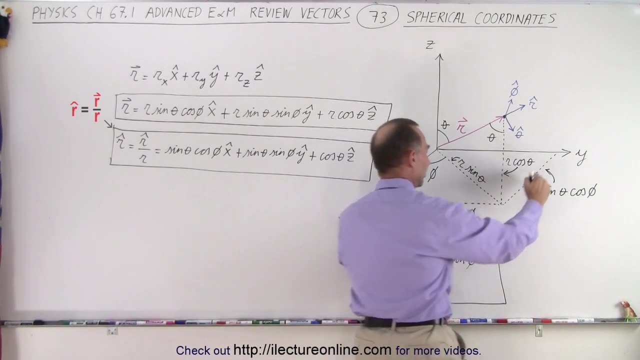 and now we have the distance from the xy plane up to that point in the z direction. So we have three distances. This is the x-distance, oh sorry, this is the y-distance. this is the x-distance. this is the z-distance. And how do we represent those? Well, take a look. Here we have the. 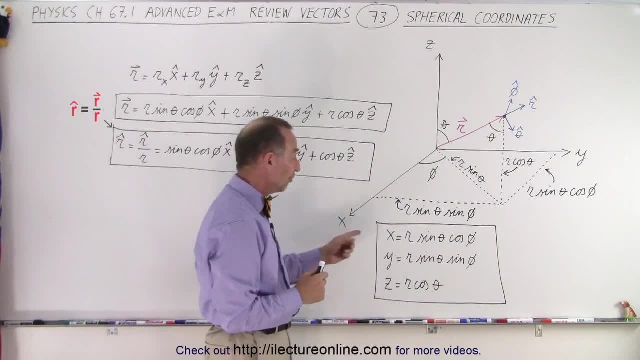 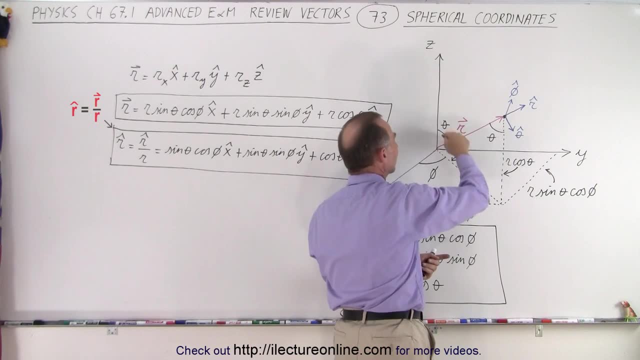 equations. but where do those equations come from? Well, first of all, let's take a look at this one right here: z, this distance, right here. Notice, if this angle here is theta, then this must be theta as well, because notice that this is parallel to the z-axis. 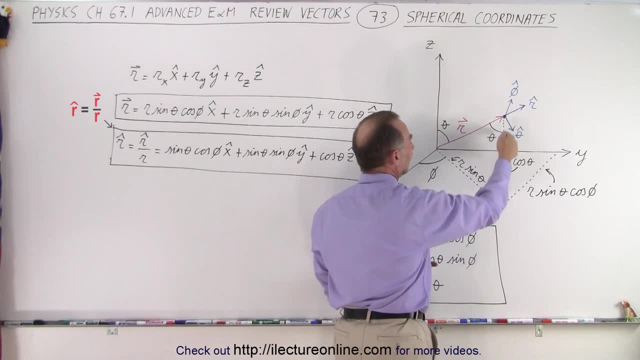 those are alternate interior angles. You can see, then, that this is adjacent to the hypotenuse, so we see a right triangle right here. This, by the way, is the right angle. Let me try to draw a right angle in the right way. There you go, there's my right angle. So. 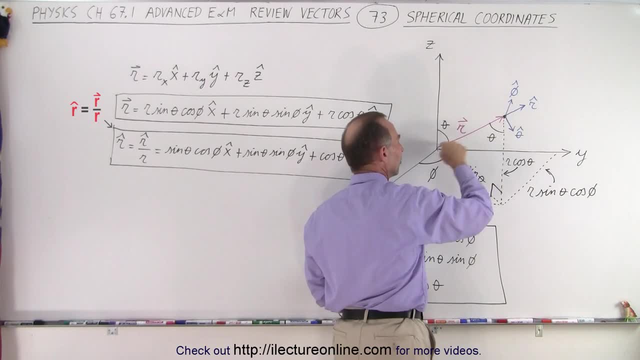 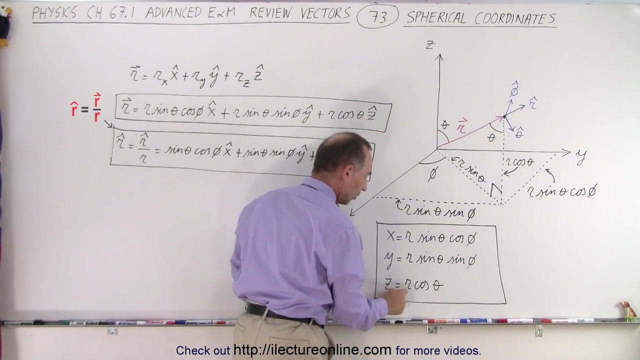 there we have it, A right angle triangle, and we can see that this is the hypotenuse of that triangle. this is the adjacent side of the angle theta. so therefore this distance z is equal to the hypotenuse r. the magnitude is r and times the cosine of the angle theta, So z is equal. 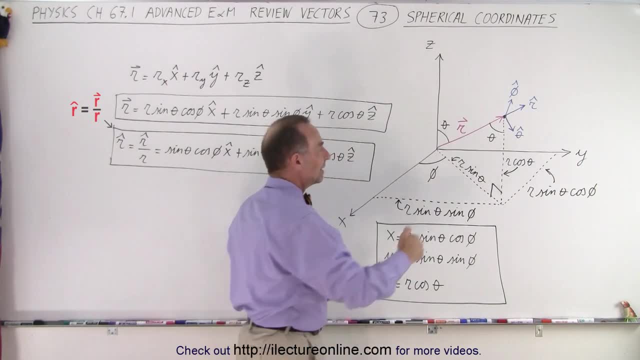 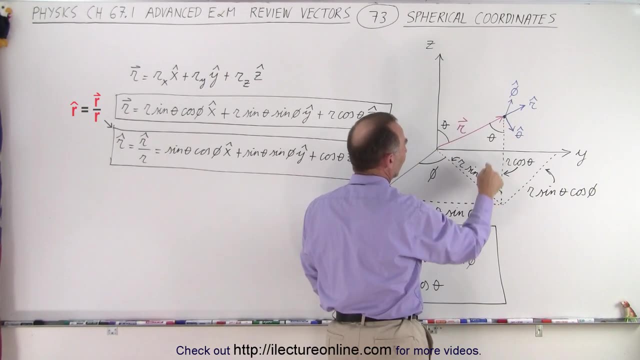 r times the cosine of theta. Now, if we take this and we project that straight down at the xy plane, what is this distance right here? Now notice that this is opposite to the angle theta. so again we have the hypotenuse of the triangle and we multiply: it times the sine of theta. 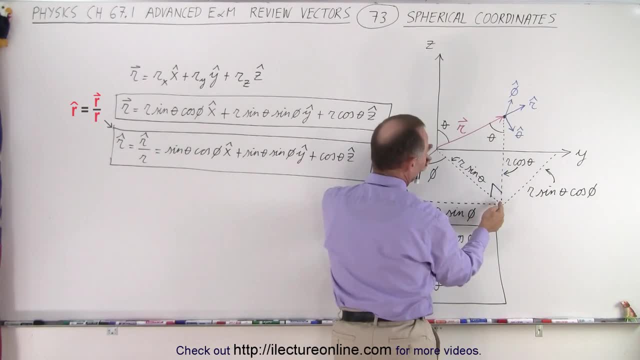 because it's the opposite side to the angle theta. So this distance here is r sine theta. Now, relative to that, we have another right triangle. Where's our right triangle? Well, let's see here: Right triangle, right triangle. that would be this right here. 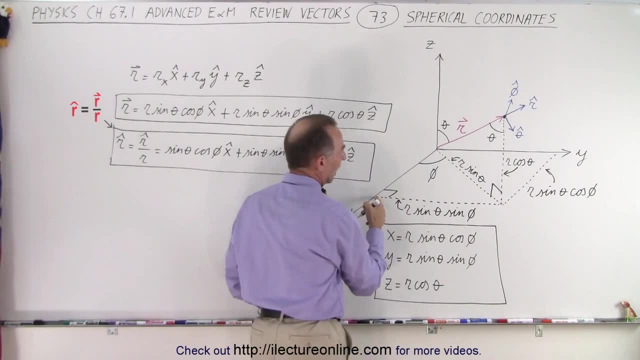 This here is a right angle, And notice that here we have a right angle, the angle phi, which is adjacent to this side right here. and now we need to know this side right here which is opposite the angle phi, and that, of course, is the y distance. so we say y is equal to this, essentially, all right. so where's the 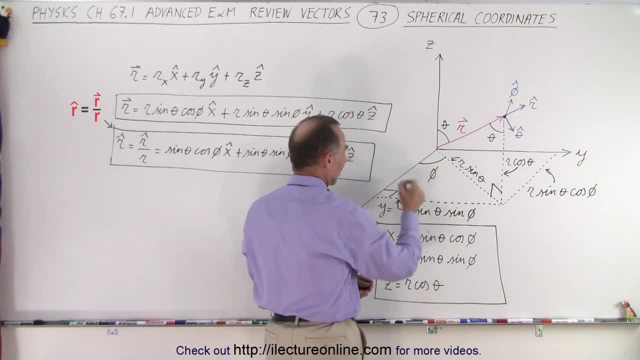 hypotenuse. the hypotenuse is here. here are the two sides: the X distance and the Y distance are the two sides. this is the hypotenuse, and so to find this distance, we take the hypotenuse and multiply times the sine of this angle, because 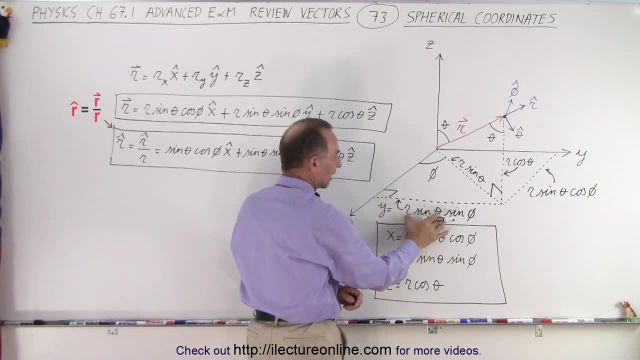 it's. this side is opposite angle, so it's the hypotenuse R sine theta times the sine of the angle. phi gives us the Y distance right here. hopefully that makes sense. now we need to know the X distance right here, which is the same as this: 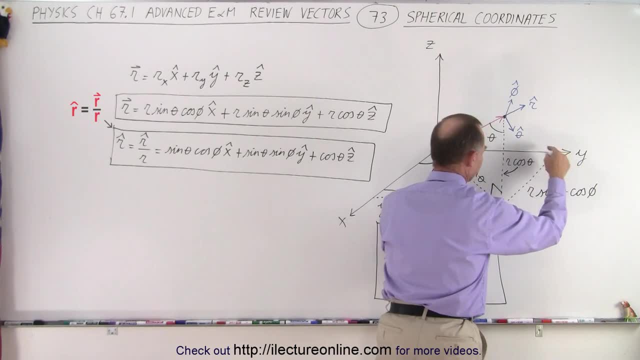 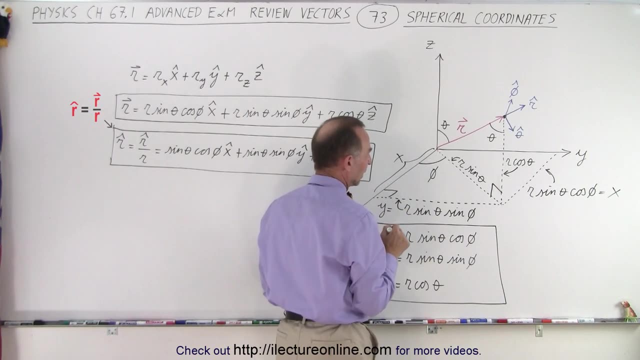 distance right here. so this here is the same as this here. so this is your X distance and so that right here would be your X distance as well. now notice that's adjacent the angle phi and we have the hypotenuse r sine theta. so x is equal to the hypotenuse r sine theta times the 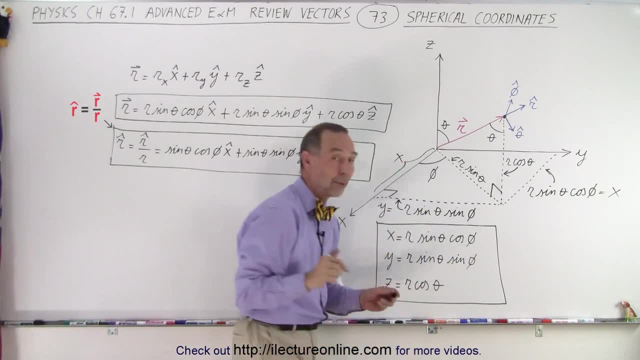 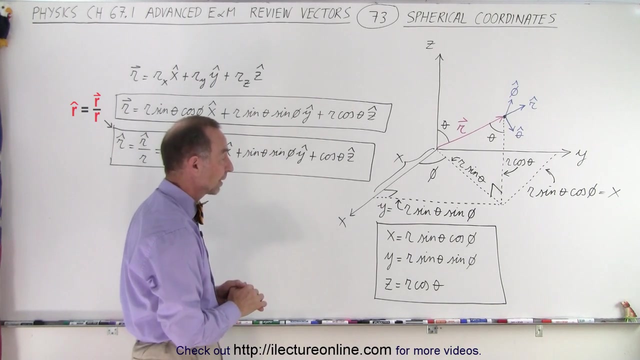 cosine of the angle phi, because it's adjacent to the angle phi. now we have an expression for x, y, z, the x-coordinate, the y-coordinate and the z-coordinate of a point in space in terms of r, theta and phi, according to these equations right here, and you can see where those equations came from. and finally, we want: 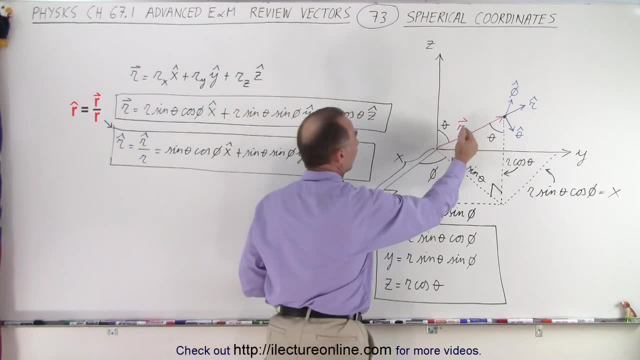 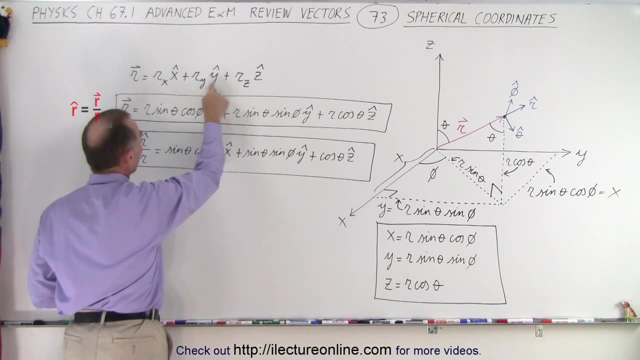 to be able to then express the r vector in terms of x, y and z coordinates, and so you can say that the r vector is the x component, the y component, the z component in the X to Y and z direction. so how do we define the x component of? 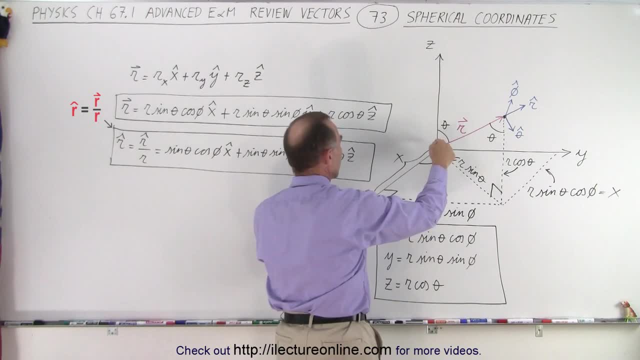 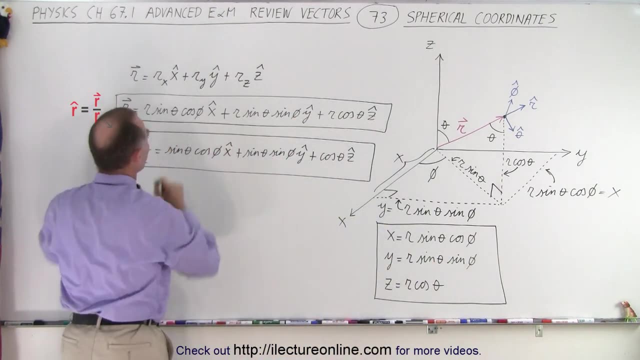 R. well, it is R projected onto the x-axis. that's this X, right here, and so the X components are sine theta, cosine phi, which is right here. then we project our vector on to the y axis. that's this distance we're over here, and that's the y-axis. so these two are the x-axis and that's the. 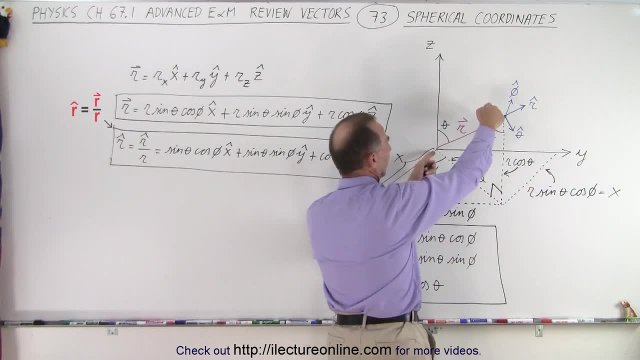 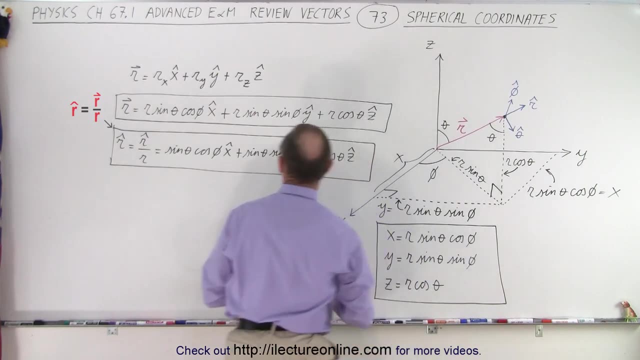 Oh, x-axis right here, which is this right here? Then we project r onto the y-axis, which gives us this distance right here: r sine theta, sine phi, That goes in here, that's the y component. And then, finally, we project r vector onto the z-axis. we get this distance right here, so we get r times the cosine of theta. 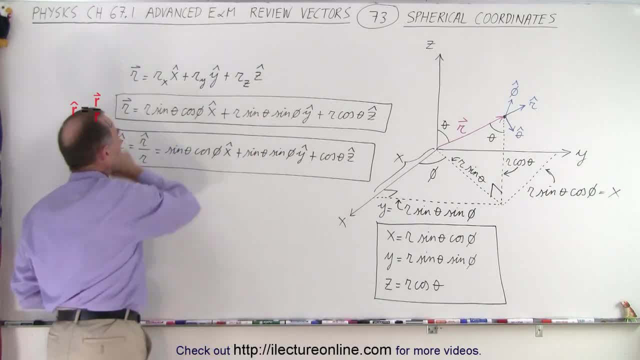 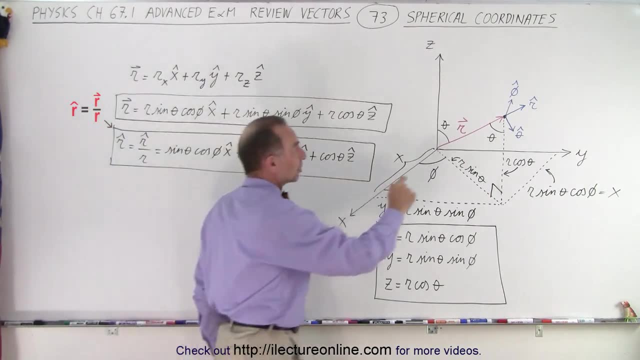 So we have the x, the y and the z components of the vector r, And that's how we denote the vector r in terms of the x, y and z components. And then, if you want to find the unit vector r right here, the unit vector r, we simply take r and divide it by its magnitude. 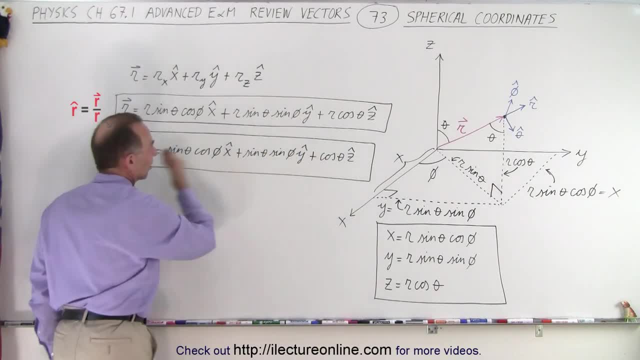 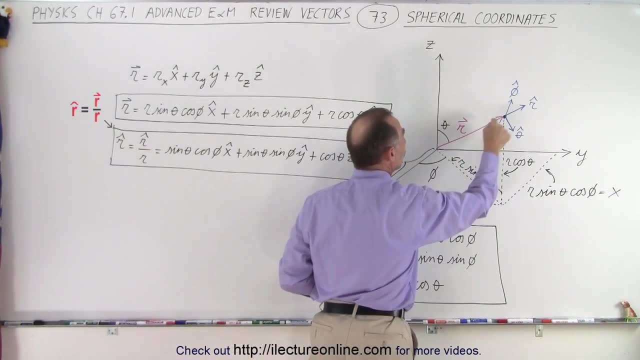 which means that all the r's cancel out and you're just left with this. This is the definition of the unit vector pointing in the direction, the same direction as the r vector: from the origin to any point in space. Now, what about the phi and the theta unit vectors? 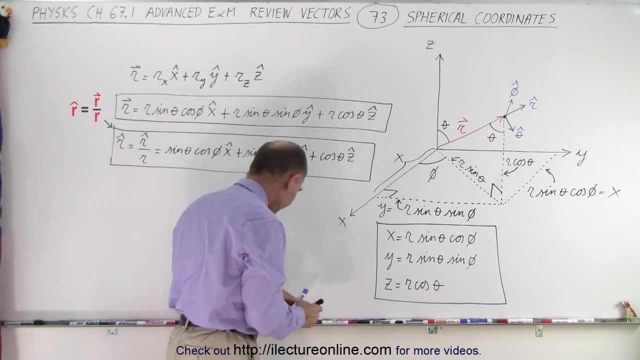 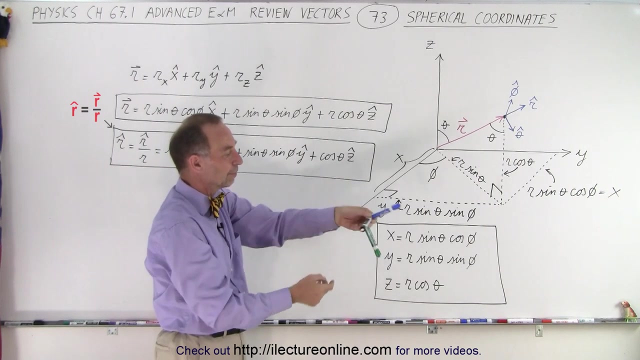 What direction do they point into? So let me try to show that I need three of these markers. So let me try to show what that looks like. So notice that these three markers are all perpendicular to one another right. There's 90 degree angles between all of them. 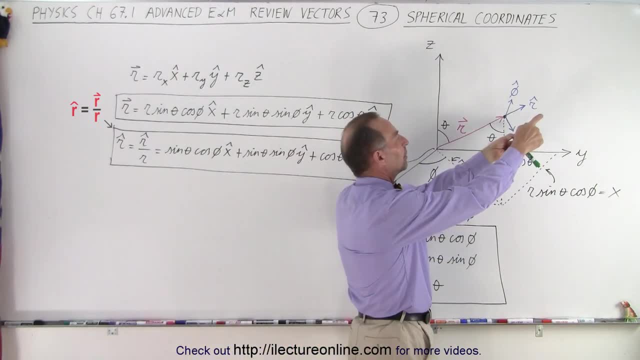 All right. so now, if I imagine that the black marker right here is the r unit vector, then the blue marker here is the phi unit vector and the green marker here is the theta unit vector. So notice that they all are perpendicular to each other. 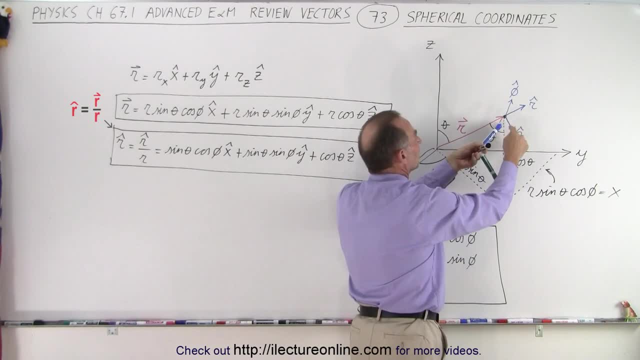 So notice that there's a 90 degree angle between r and theta, There's a 90 degree angle between r and phi and there's a 90 degree angle between theta and phi. So they're all kind of located like this. It's hard to draw that on the board, of course. 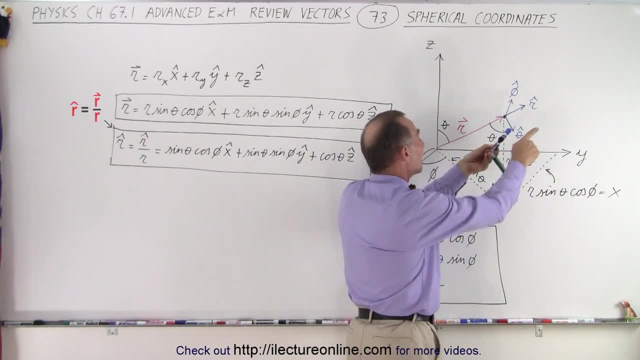 But if you use a little bit of imagination, you can see that the theta vector points at a 90 degree angle relative to the r vector. Wherever the r vector is pointed, no matter which way it's pointed, notice that the theta vector- I'm sorry, the phi vector. 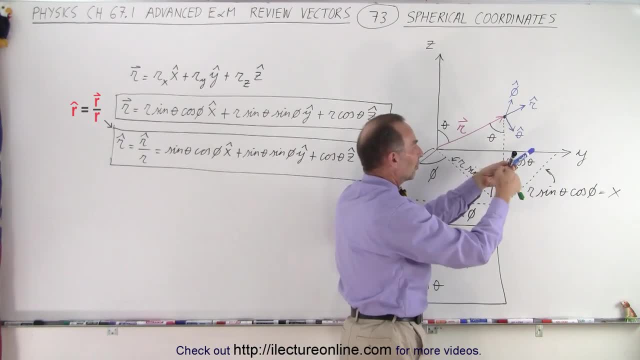 phi vector is pointing away like this, And then the theta vector is pointing, Okay, Okay, Okay, pointing straight down again. there's a 90 degree angle between r and the theta unit vector. r unit vector points directly in the same direction as the r vector and the phi unit vector points at 90.